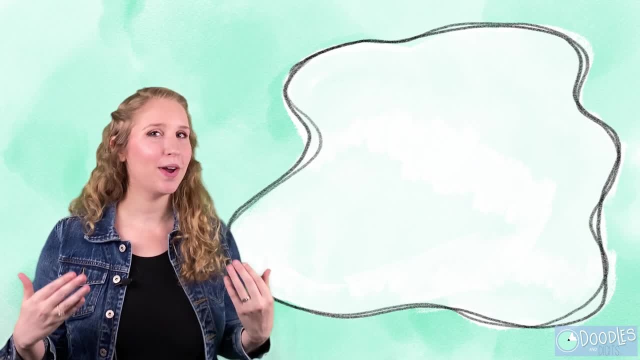 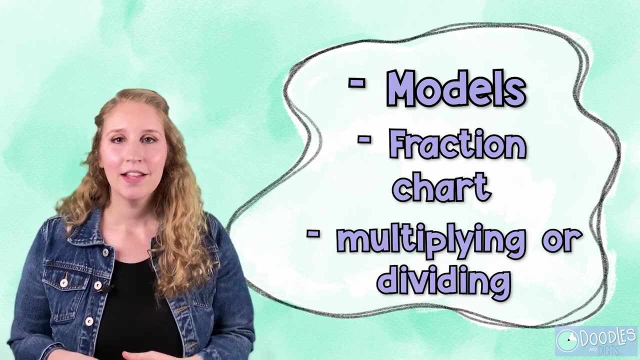 fraction and use that measurement instead. Alright, now that we know what equivalent fractions are, Wow, we find them. There are actually a few different ways that you can find equivalent fractions. Let's first look at this. right here, We're going to look at some models. 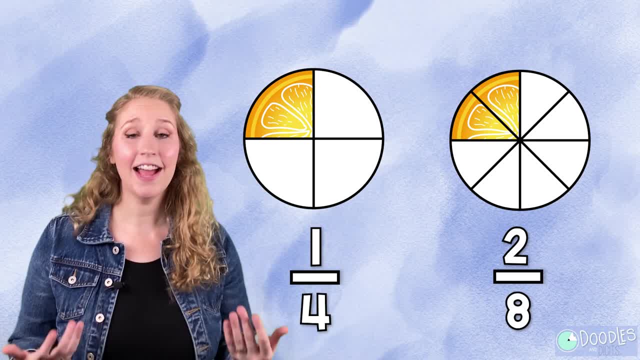 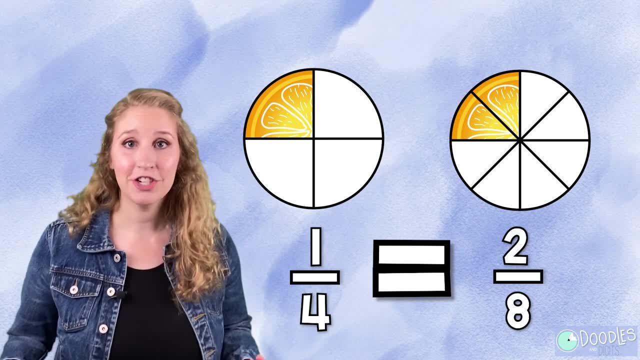 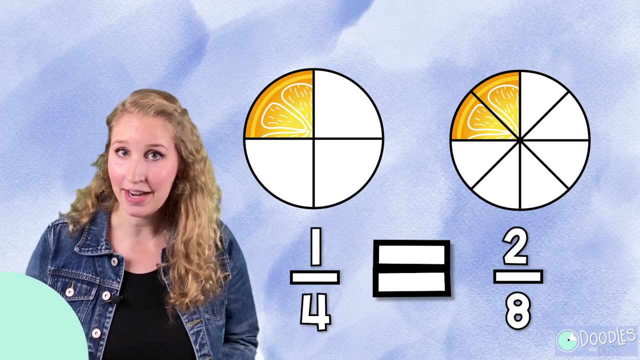 What do you notice is going on? That's right. You can actually look at a model and cut it into more pieces to find a different fraction. When you cut that same model into different pieces, you're actually finding an equivalent amount with a different denominator. This is a fraction chart. 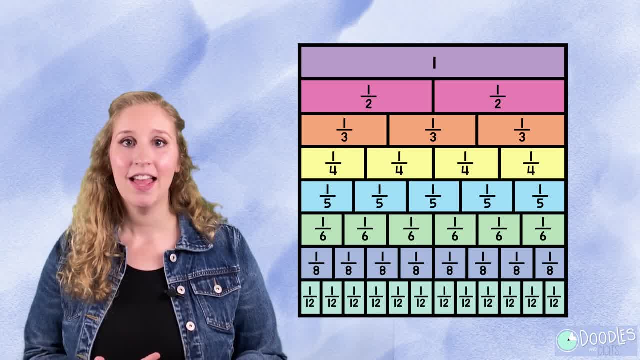 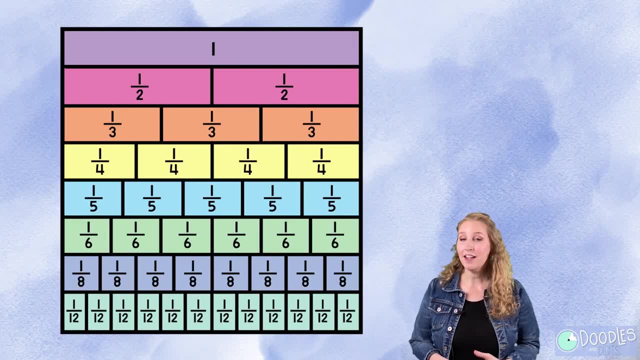 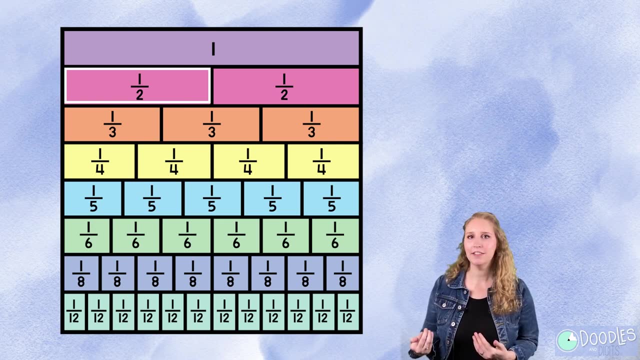 A fraction chart is a great way to find equivalent fractions and to see how fractions compare to one another. Let's look at this one right here. If we were trying to find a few equivalent fractions to one-half, what do you notice? Do you see any that are close to one-half? Do we see any that are exactly one-half? 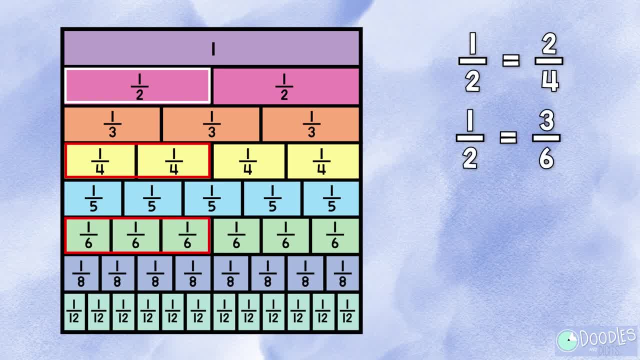 One-half is equivalent to two-fourths. It's also equivalent to three-sixths. One-half is equivalent to twoودths, Also equivalent to three-sixths. Do you know how that was compared? motions include molto ovatoe and we can't know how that's compared. 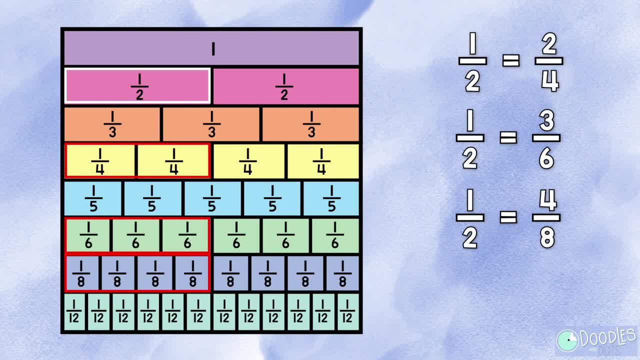 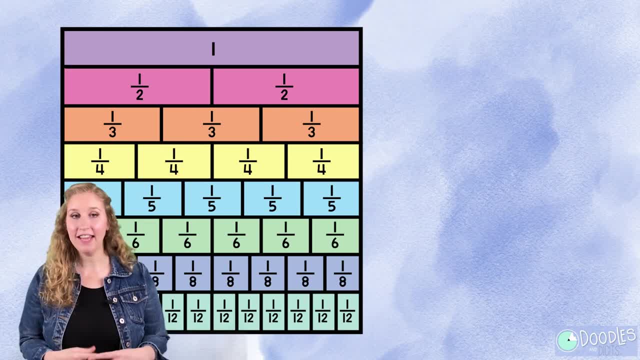 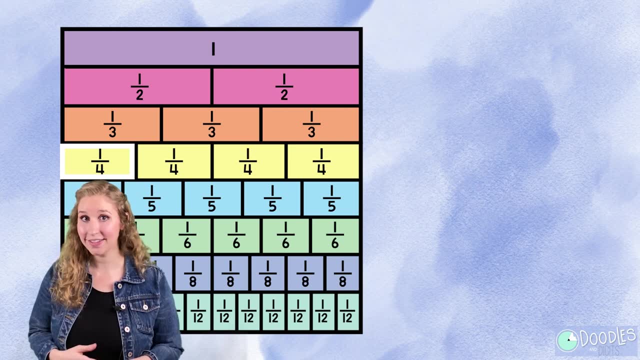 1 half is equivalent to 4 eighths and finally, 1 half is equivalent to 6 twelfths. There are so many fractions equivalent to 1 half on this chart. Alright, now that we have found equivalent fractions to 1 half, can you find a couple equivalent fractions to 1 fourth? 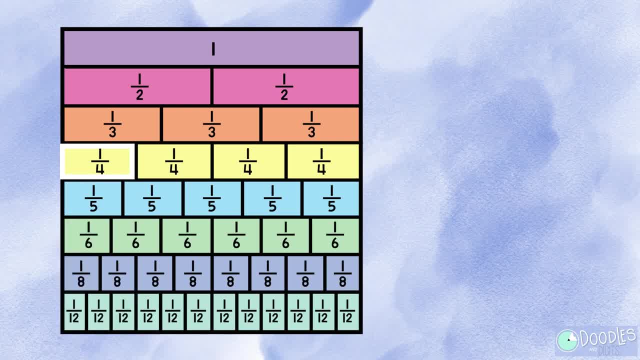 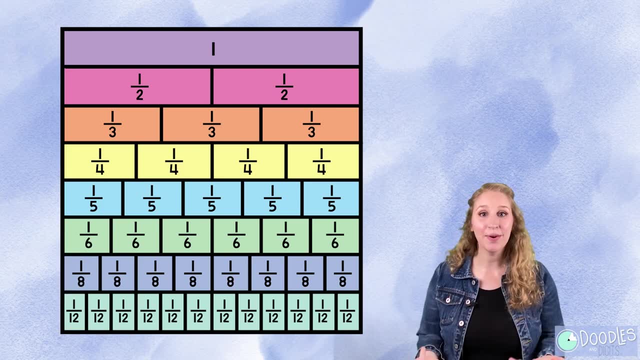 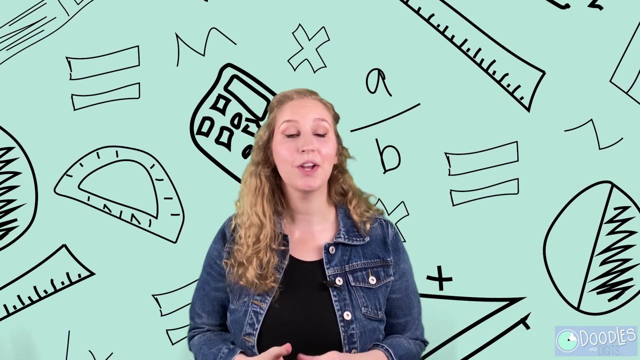 1. fourth is equivalent to 2 eighths. 1. fourth is also equivalent to 3 twelfths. Again, a fraction chart is a great way to make math visual, so you can actually see what two fractions are the same. You can also find equivalent fractions by multiplying or dividing the numerator and the denominator by the same number. 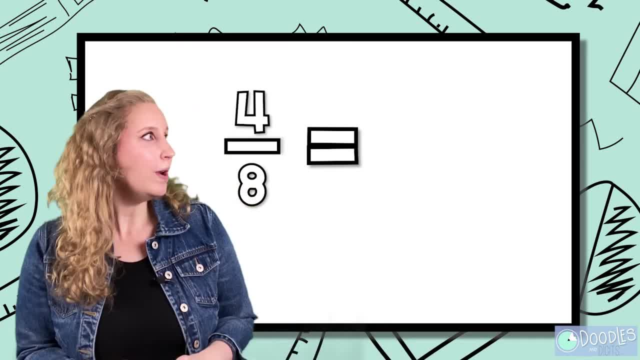 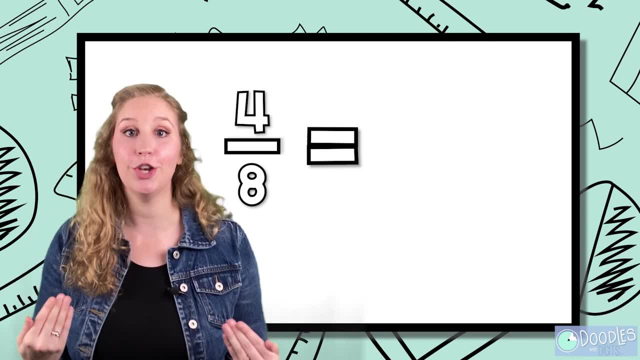 Let's look at this problem right here. So when we look at this fraction, we're going to multiply the numerator and the denominator by the same number, So let's say 2.. We're going to multiply the numerator by 2 and the denominator by 2.. 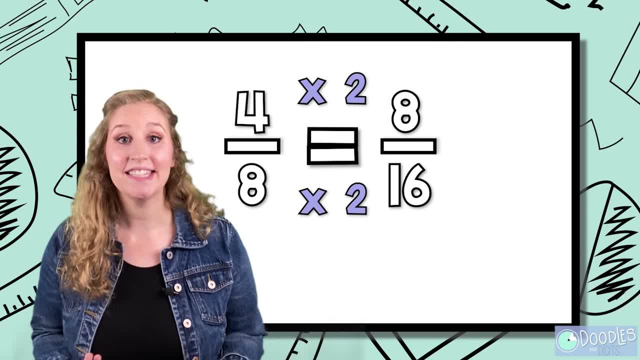 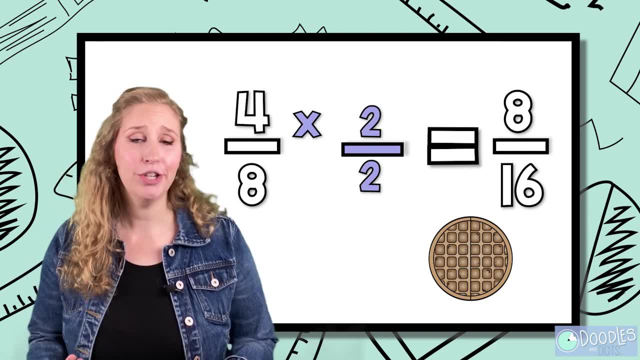 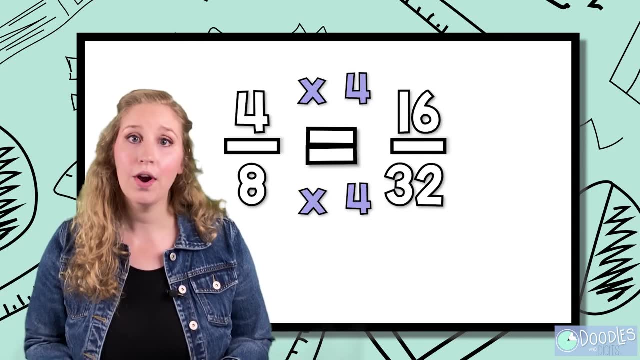 When you multiply the numerator and denominator by the same number, you are actually multiplying by one whole. Look, 2 over 2 is actually 1.. So you can multiply by 3.. 3 over 3.. 4 over 4..